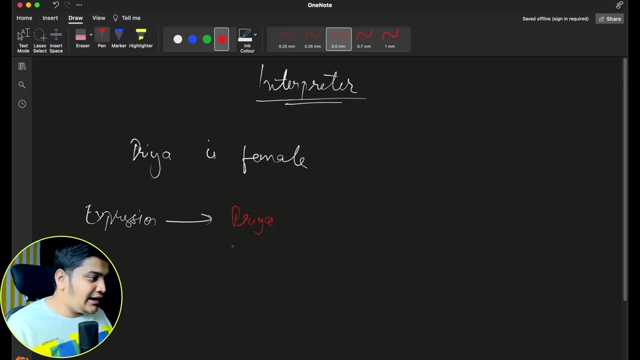 if that particular expression contains Priya and it also contains female, Okay, That means that Priya is female. Okay, Now, this is the expression. Now, if I am passing this thing, Priya here, Priya is a female here within this expression. it will check. Okay, This particular expression. 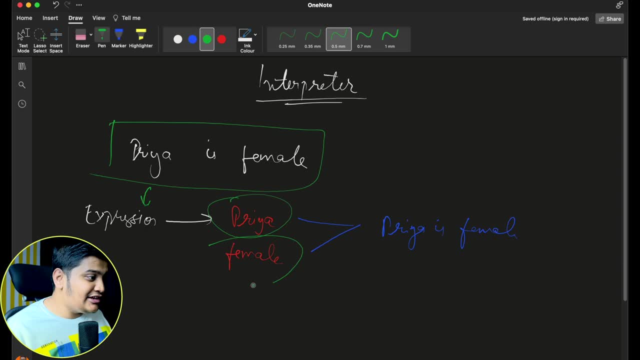 has Priya as well. This particular expression has female as well. So it's checking both the things. This is also true And this is also true, right? So both the things are true. That means the entire expression is a female. So I can say it's an and expression. I can define this as an and expression. 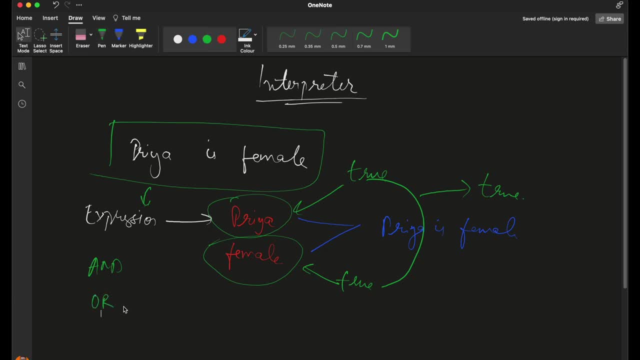 I can define one more as an or expression as well. I can define a normal expression as well, just to identify that particular sentence is true or not. So there are different ways that I can define the expression for the interpreter. So interpreter is nothing but an expression. 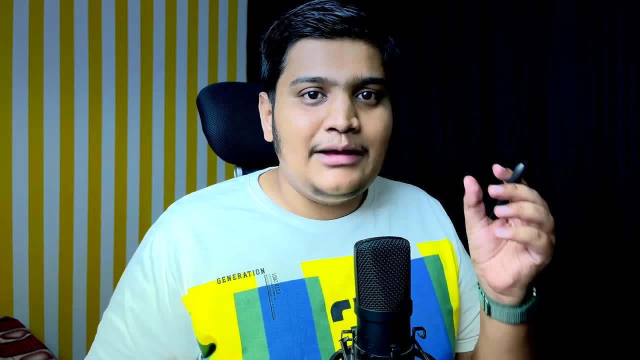 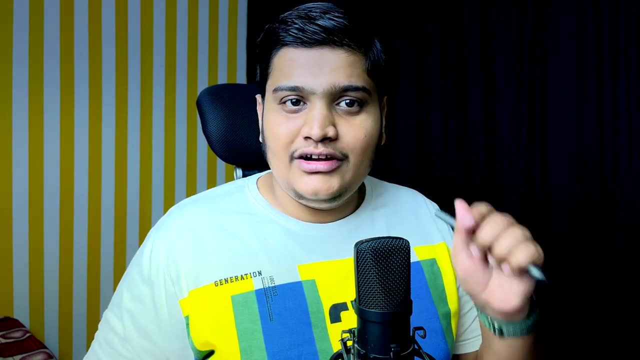 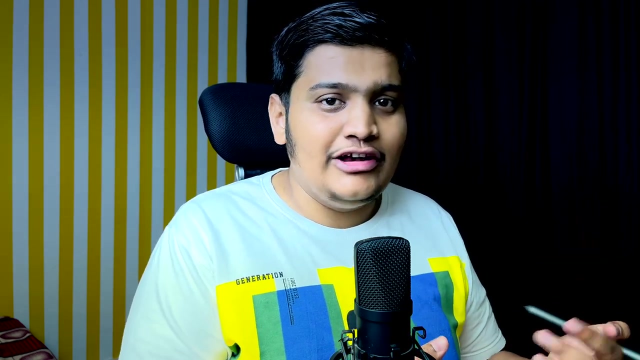 evaluation where different types of expression is passed and based on the logic, that expression has been evaluated for a interpreter. Okay, So interpreter is nothing but an evaluation of the expression and it will just return what actually that value is: It's a positive value or negative value. So, ideally, if you are working for any language, 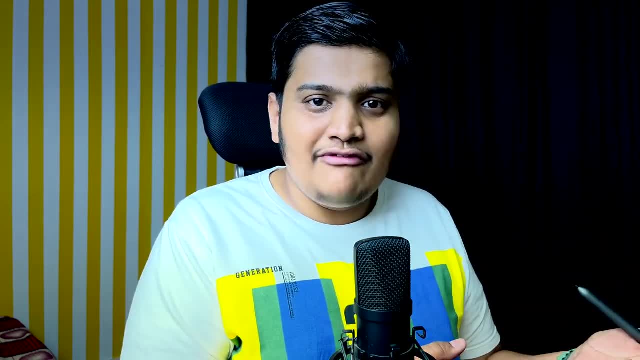 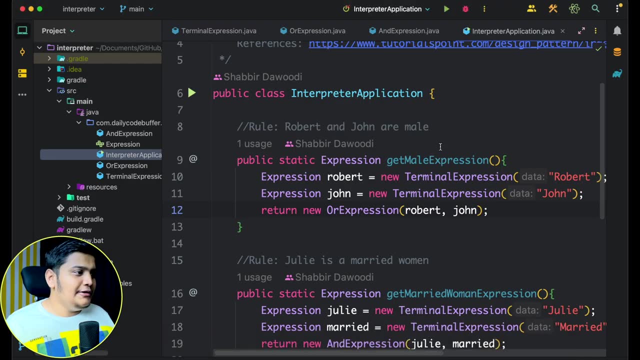 or interpreter. that's how it has been done. Okay, So that's the behavior of it. And let's understand with the code as well, like how that particular behavior has been defined. So if I go to the code here, okay, You can see that this is the particular example of the interpreter. 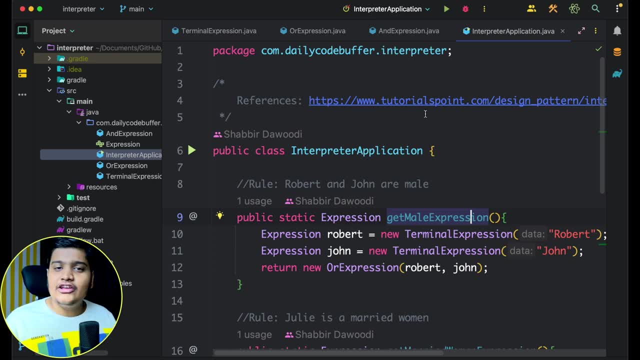 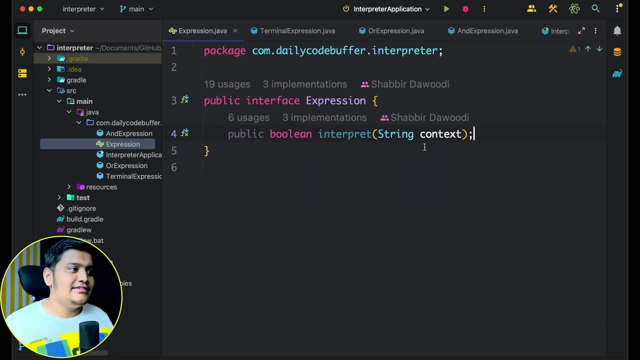 I've taken this example from the tutorials point. I have added the link for that as well. You can go through it and you can read about it it more there as well. Now, currently, you can see that what I have done is I have defined one interface that 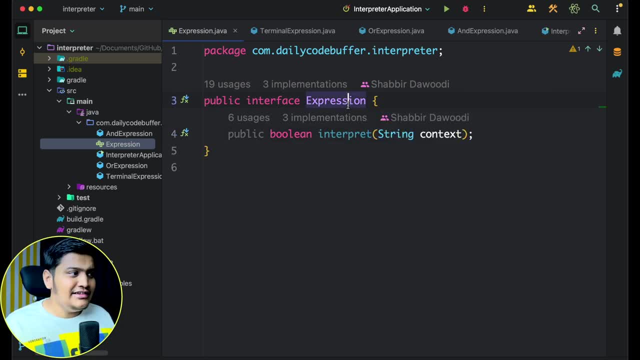 is the expression interface. okay, and within this expression interface, I have defined one method, that is the interpret method. So, whatever the context that I give here, that context needs to be interpreted by this method, and this method will return either true or false. that's the Boolean method. okay, that's. 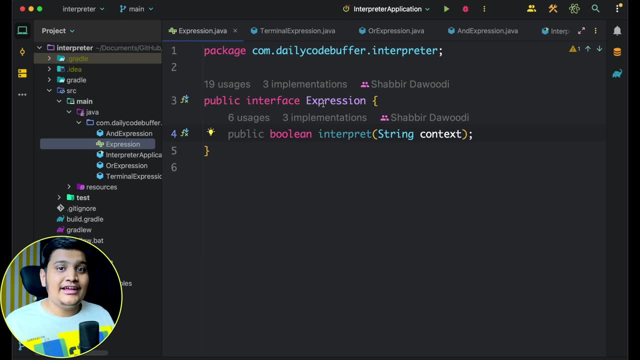 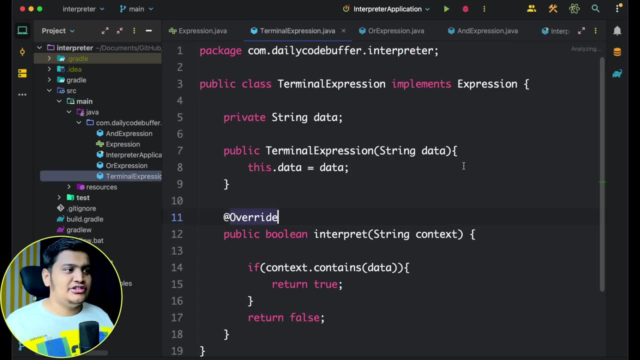 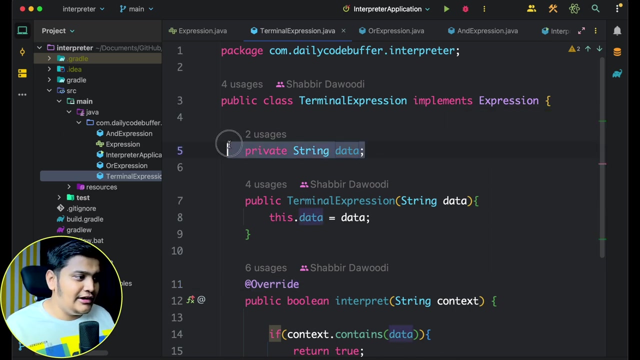 the simple job of the expression here. Now, this expression can be implemented by the different types of expression. okay, suppose let's take one example. that's the terminal expression. okay, that's the basic expression here. that is implementing expression, and what it does have is it has the data as well. okay, 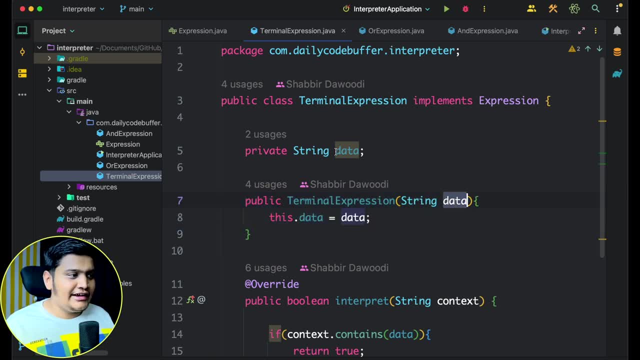 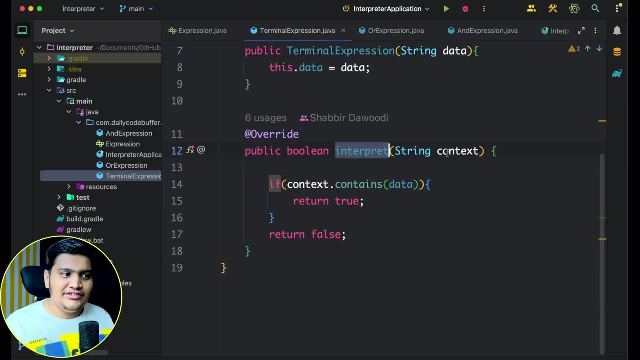 and here you can see that I have created the constructor here which is taking the data and it is setting here. Now I have implemented the interpret method, which is part of the expression here- interpret- and which is taking the context. And what I am doing is: 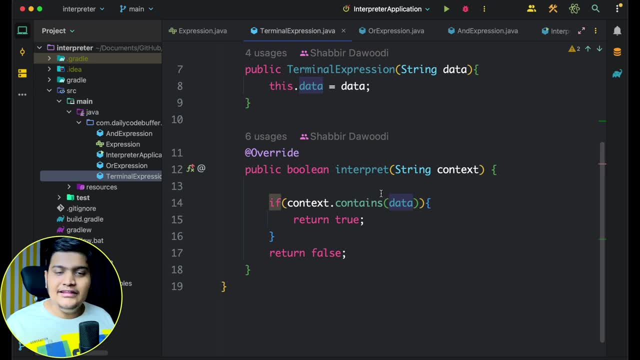 If that context contains the data, then that means that's a true. otherwise it's a false. so that means if I am adding the terminal expression as Priya and I am adding Priya as a female, that means it was able to find the Priya within that particular context. so 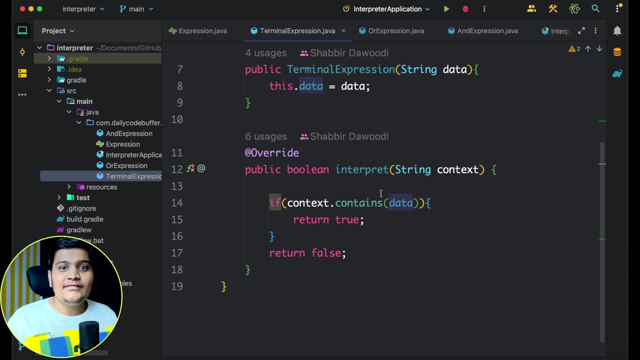 it will return true that. okay, whatever the data that you have as an expression, that is part of the context as well. okay, so that will return true, else return false. so that's one of the terminal expression. let's see one and expression as well. So within this and expression: 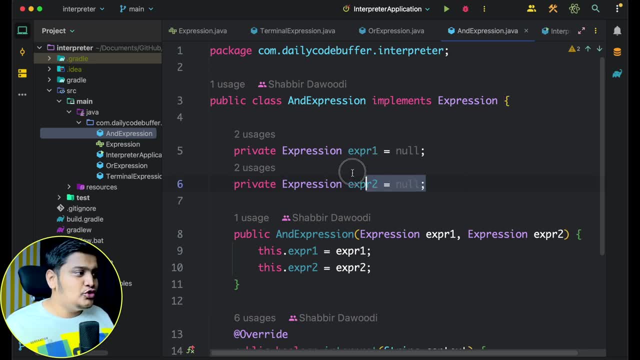 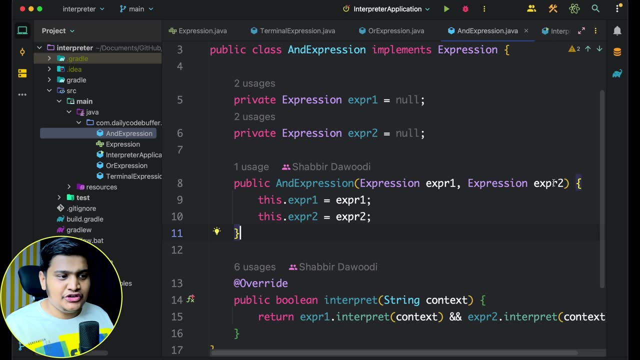 You can see that it is implementing expression and it has two properties, that is, expression one and expression two, and this is the constructor here that I have defined, which is taking expression and one and expression two, and it is setting the values here, and I have added the interpret. 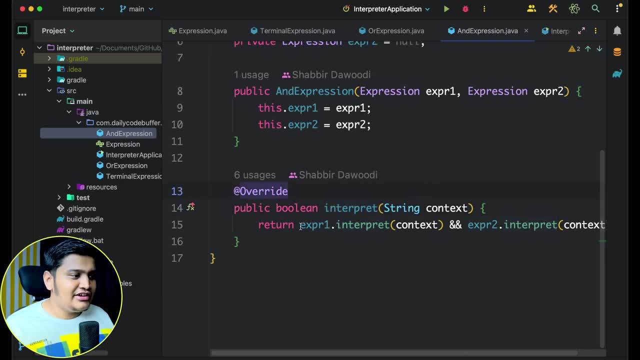 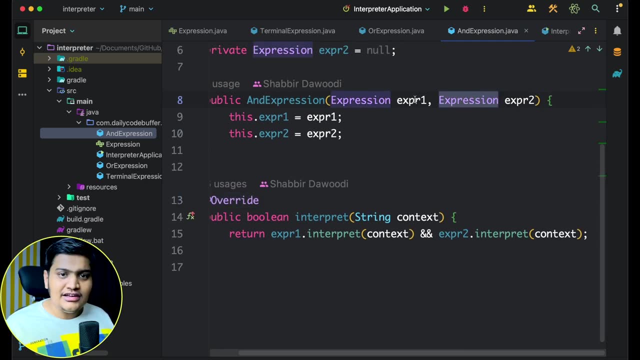 method here as well. now, what interpret method is doing is it is checking that expression. one dot interpret. I am just interpreting this expression because this expression is also been interpreted. it's a interface, right? so if that is returning true and the second one is also returning true, 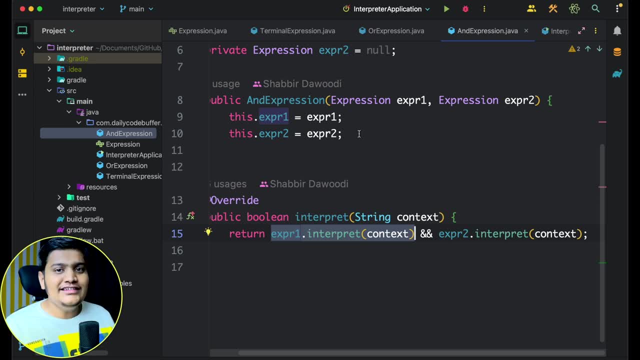 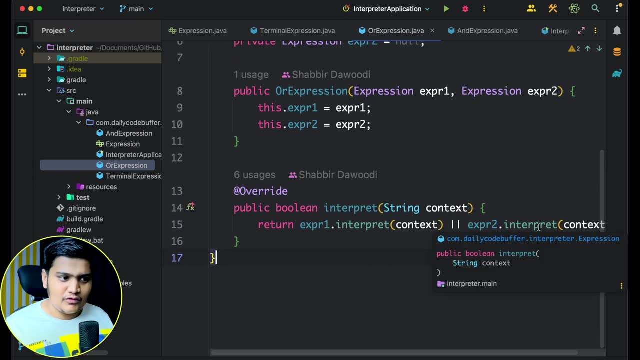 That means both are returning true, that's true. otherwise it's a false. so that's it and expression for me. similarly, our expression would be either this or this: okay, so I will just define this expressions here now, when I am going to call this, you can see this is: 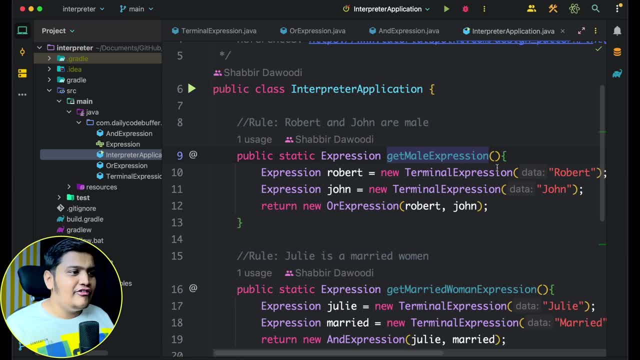 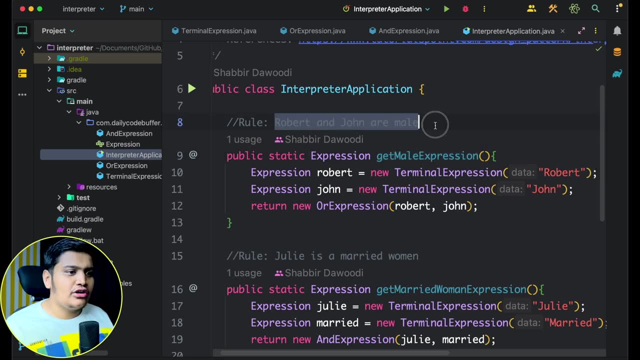 the interpret application that I have defined here and here I have defined different expressions. so here you can see that I have defined get male expression, okay, and here I have defined that Robert and John are male and here there are two expressions: That terminal expression contains Robert and terminal expression contains John, and if 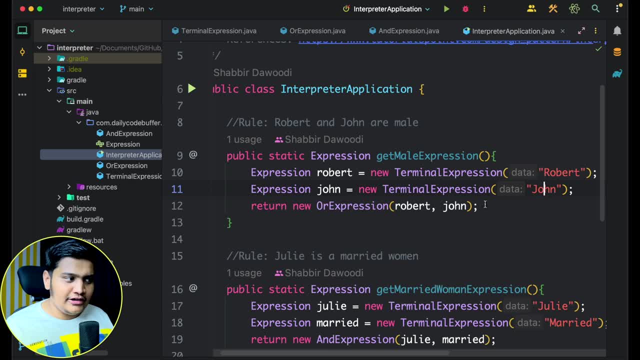 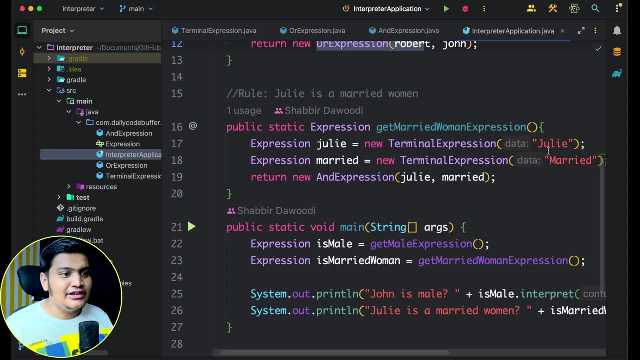 we are passing these two values- Robert or John- within the or expression, it will return true, okay. similarly, I have one more that is get married woman expression. so Julie and married. these are the two different context that I have provided, data I have provided in the terminal and we have called the and expression. if we are getting both the values, 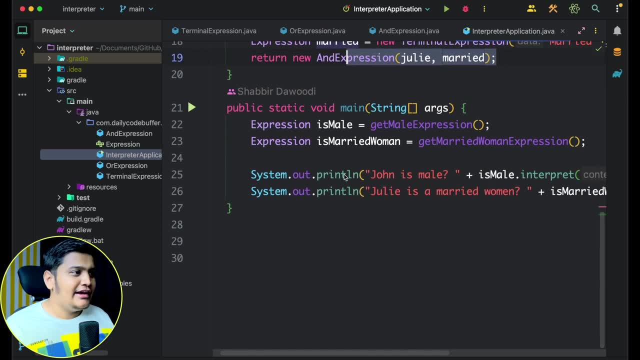 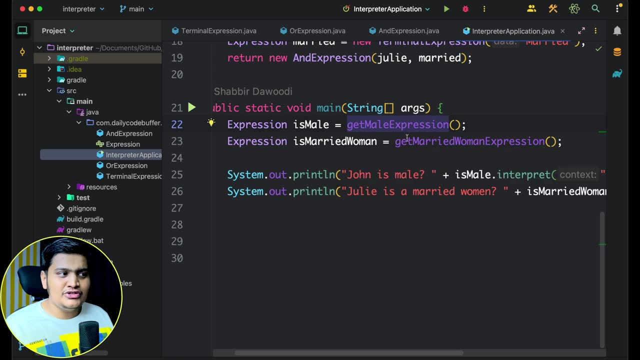 Julie and married, then this will return true. Okay, And yeah, this is our main method, where we are actually calling it. so your expression is male equals to get male expression and expression is married woman equals to get married woman expression. okay, and I'm just trying to print this: John is male and I'm 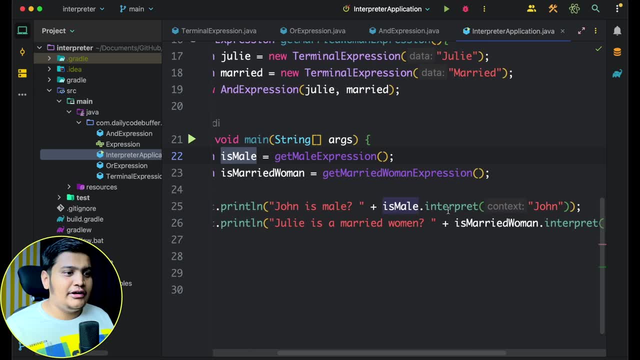 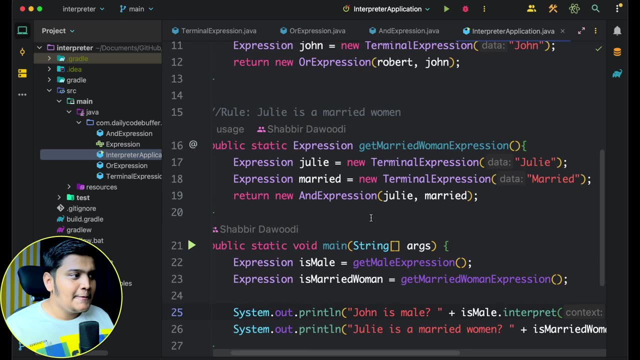 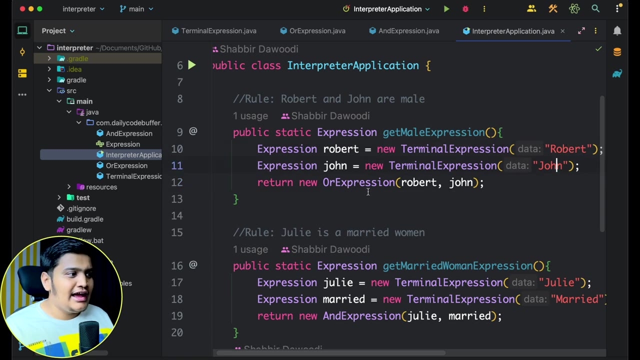 just trying to call is male. this is the expression. dot interpret what is trying to interpret: John. now we are passing John as the context. this context will be interpreted by this expression. okay, and within this expression there are two values: Robert and John. This is the or expression. so whenever there is or expression, this expression expression. 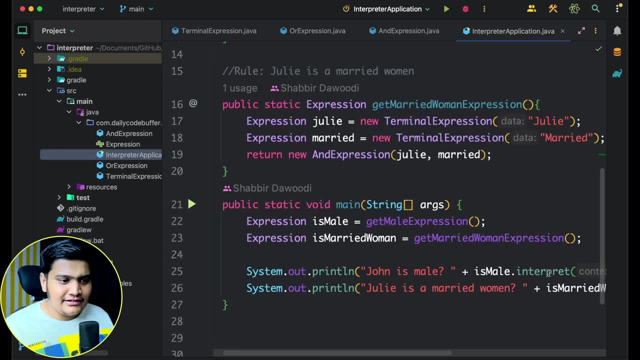 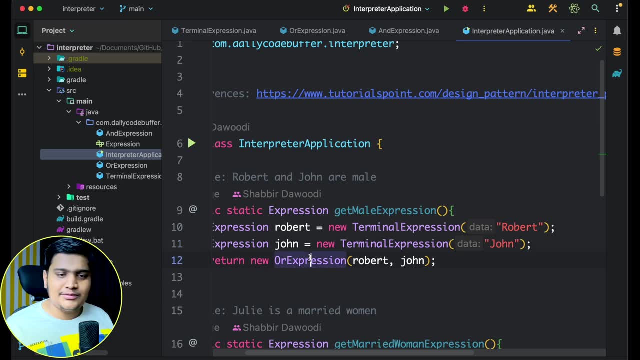 has been called. it will check. okay, we have data as John. this is the context that we have provided and within that context, we have two data, Robert and John, and we are calling or expression here. so this or expression will be true and it will return true here. okay. 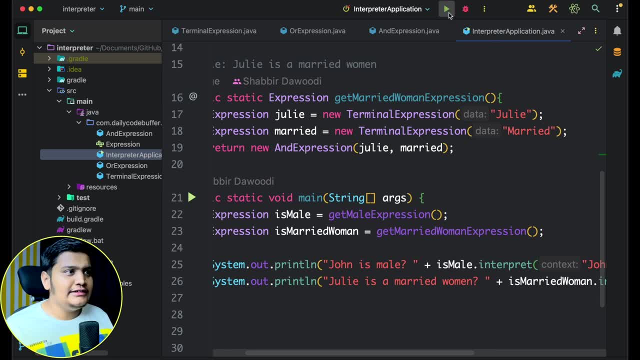 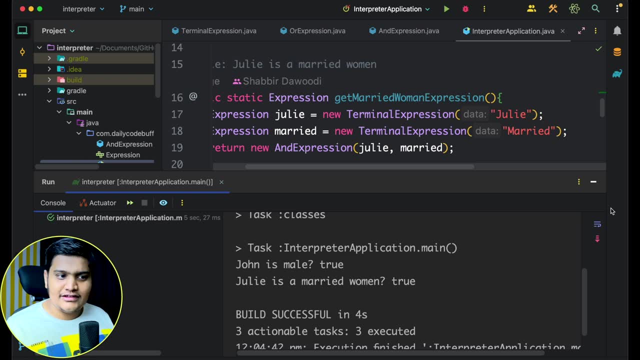 that's the way. similar for the Julie is a married woman. so if we run this, you can see that we are getting the same thing: that John is male, Yes. Julie is a married woman, Yes. Okay, so this is how that expressions are working and this is how you will be implementing. 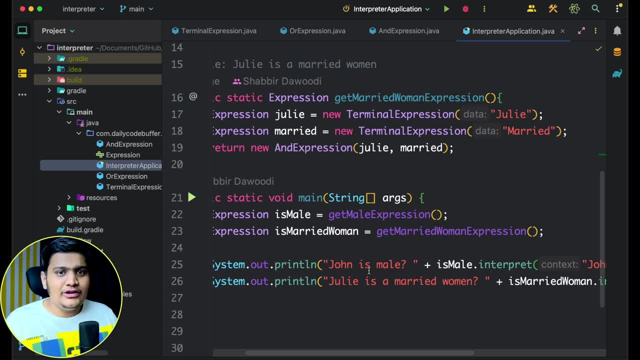 the interpreter design pattern. you can see, that is very simple. you are just defining the interface and for that interface, you are just defining the different concrete classes, and for all those concrete classes you can define different methods for defining those different expressions. okay, so for every expression you have to define like what this particular 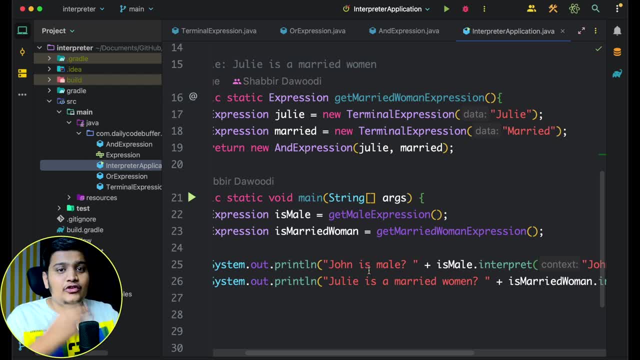 expression means that's how you define in the language as well, like you define a tree, like: if this, this, this are there, This is what it means. okay, So this is how similar in the interpreter as well. so you have to interpret each and every thing that you pass, okay? so I hope you enjoyed this tutorial. you can see it was very easy. 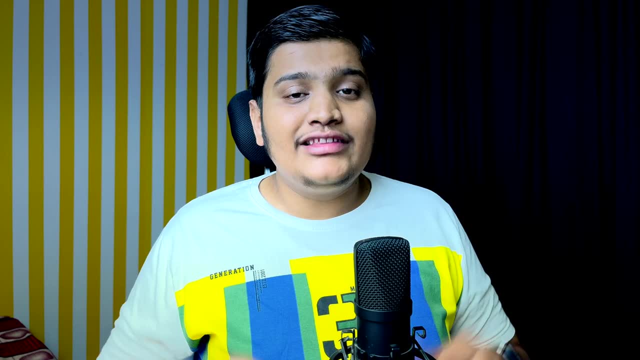 to implement and if you have any doubts regarding any of the things that we have covered, then do let me in the comment section below and, if you like this video, give us a thumbs up and subscribe to my channel for the upcoming videos. you can also click on the join button. 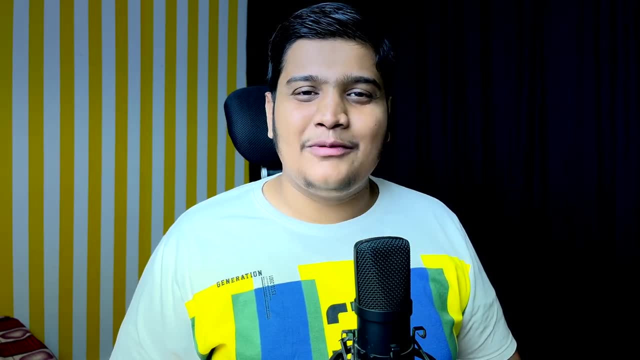 to support my channel. I will see you in the next video. till then, happy coding, bye, bye.